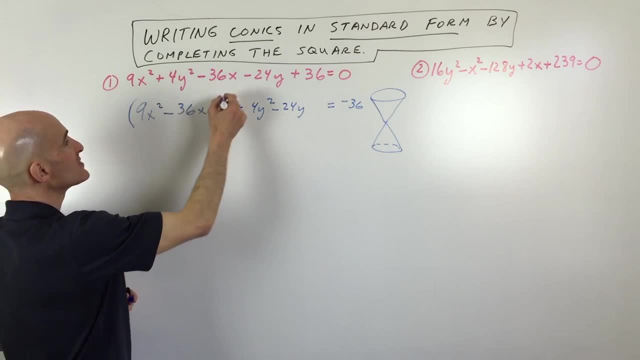 just to get it out of the way Now, what we're going to do is we're going to group these together, the x's and the y's, and we're going to factor out the leading coefficient. So if you factor out a 9 here, what we're going to have is x squared minus 4x. and if we factor out a 4 here, 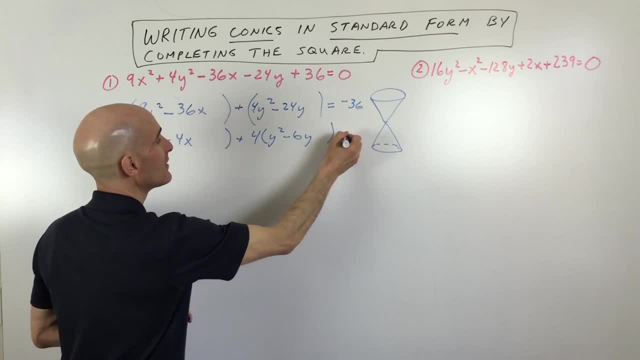 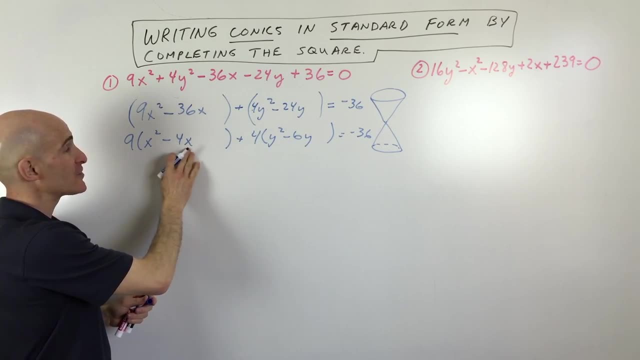 we're going to be left with y squared minus 6y equals negative 36.. Okay, Okay now what we're going to do is we're going to complete the square, and we do that by taking half of the coefficient in front of this middle term here. So half of negative 4 is negative 2,. 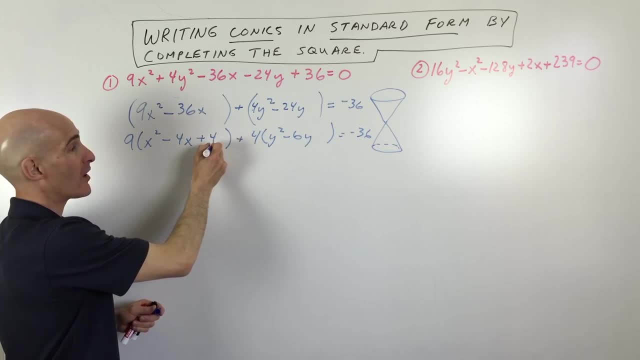 negative 2 squared is positive 4.. Okay, now, what I want you to recognize is that, because it's in parentheses, it's actually 9 times 4 that I added out of thin air. okay, 36 to the left side of this. 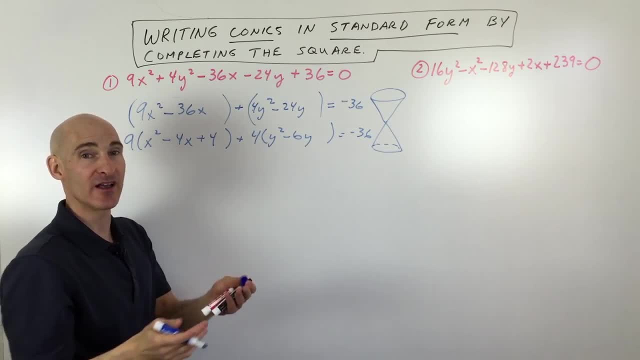 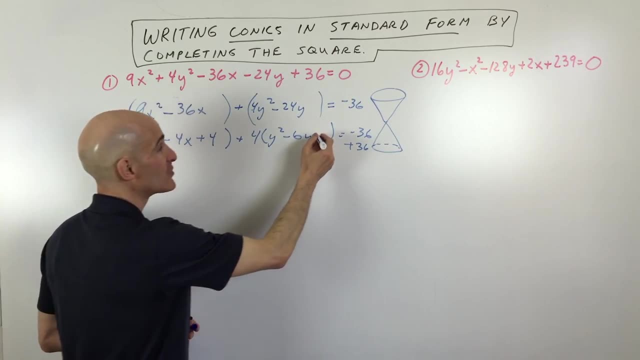 equation, I have to add 36 to the right side to keep it balanced. Okay, so let me just do that right here, plus 36.. Over here, half of negative 6 is negative 3. If we square that, we get 9.. 4 times 9 is 36.. Again, if I add: 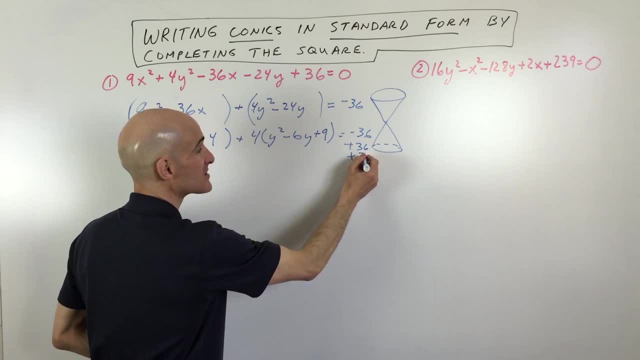 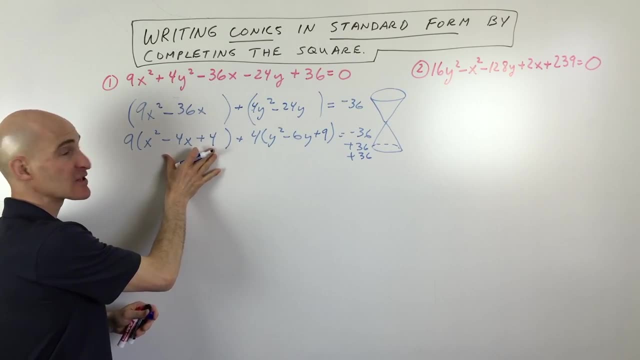 36 out of thin air to the left side, I have to add 36 to the right side to keep it balanced. Okay, so far, so good. So now we're going to factor this and the way that we've set it up, because 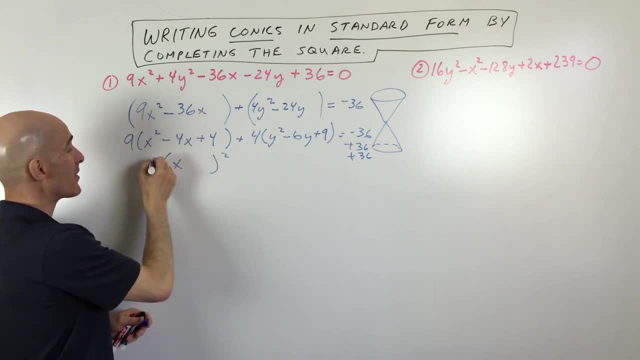 we completed the square is that this becomes a perfect square. and one thing that I tell students all the time is that you can always look at this middle coefficient and just take half of that quantity. So if it's positive, you can always look at the middle coefficient and just take half of. 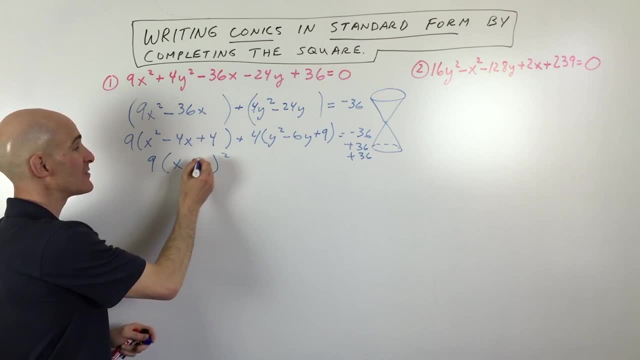 it. So if it's positive 4, this would be positive 2.. If it's negative 4, it's just going to be negative 2.. If you want to verify this, just go ahead and write x minus 2 times x minus 2,. 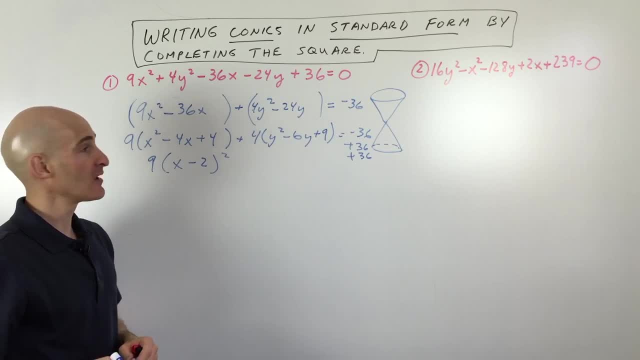 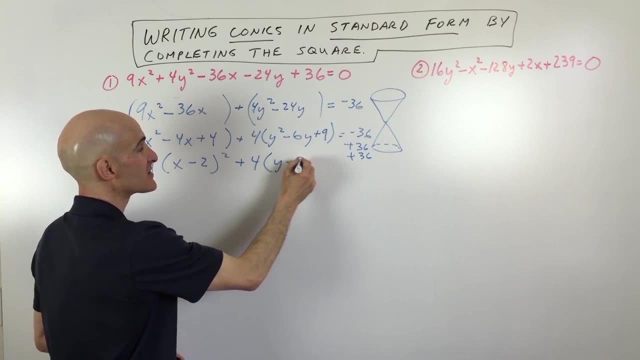 FOIL it out. multiply it out and you'll see you get back the original. but this is just a little shortcut. Same thing over here. What you can do is take half of negative 6, so that's going to be y. 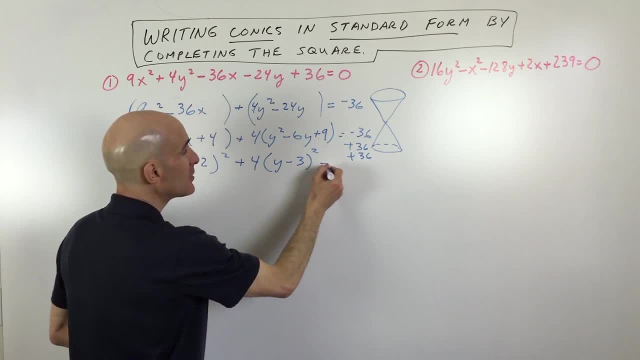 minus 3,, the quantity squared equals these 36's. cancel out, and we're just left with 36.. Okay, now what I'm going to do is I'm going to divide everything by 3, and I'm going to divide everything.